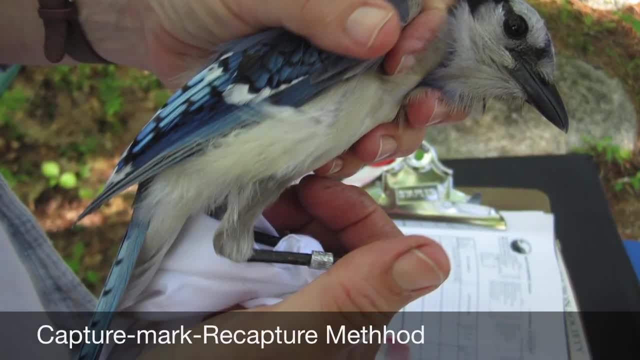 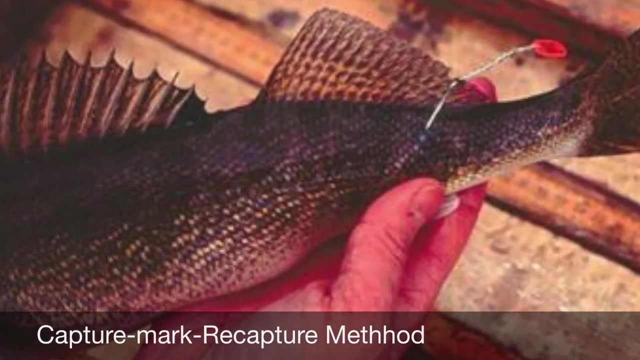 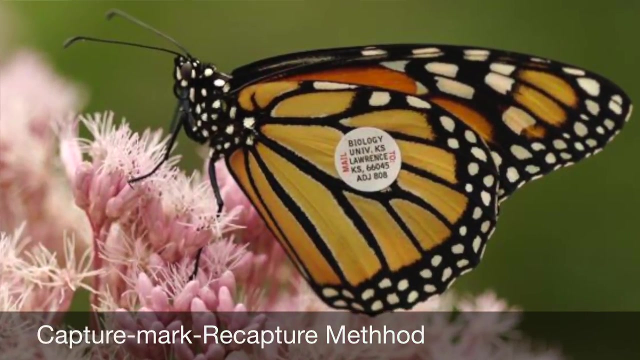 That one is relatively straightforward, where essentially what you'll do is capture a certain number in a population. You mark them or tag them, You release them back out into the wild and then what happens? It transpires later. You come back in a few weeks or months, or what have you to let them? 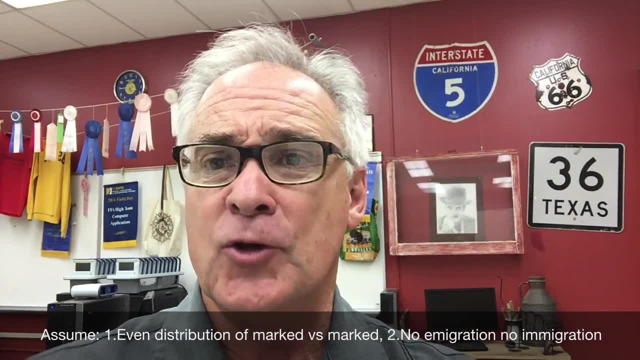 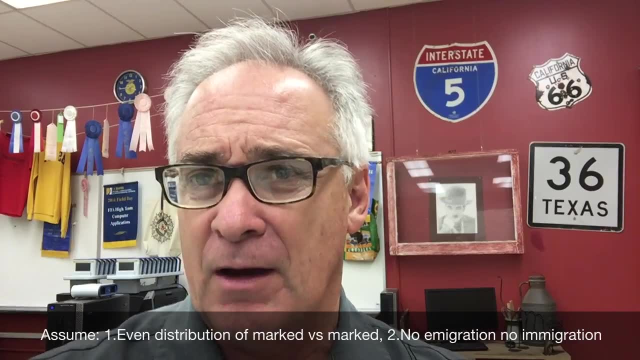 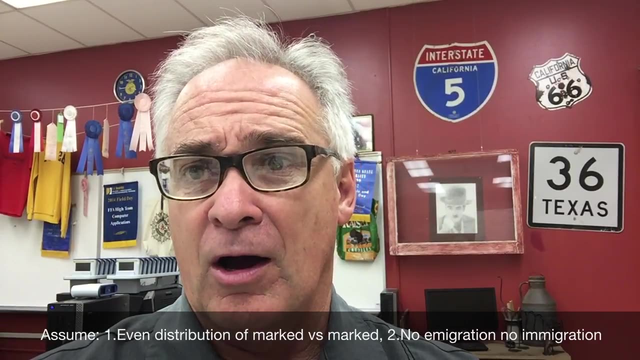 redistribute themselves in their particular environment and then you recount them And possibly you may want to do this over a period of time so that you get an estimate of approximately how many in the area. So I want to show you kind of a classic experiment today on how to do this. 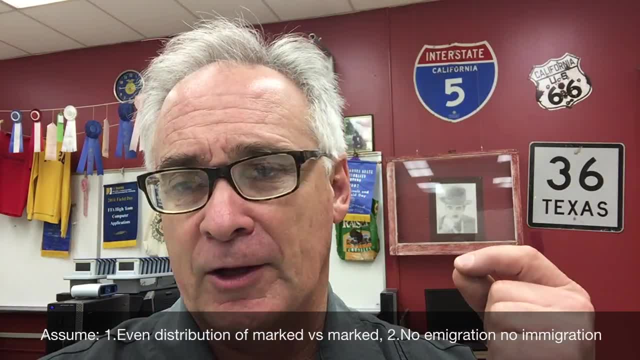 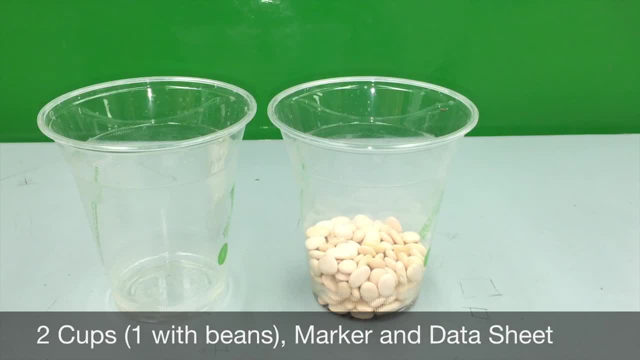 capture mark and recapture. First of all, we'll take a look at some of the materials procedure and then we'll end with you. now, All right, as far as the materials are concerned, they're pretty straightforward and simple. You'll need two plastic cups and, as you can see, 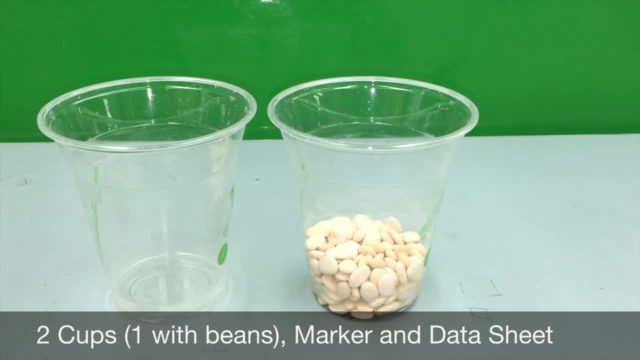 they're a quarter to half filled with some kind of white bean- Small lima beans work really well- and again- so you just want to get a half to a quarter. I've used a quarter just because for this demonstration it's a little bit easier to count. Also, you're going to need some pens. 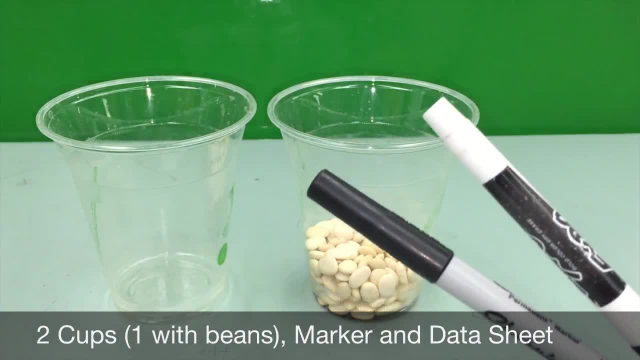 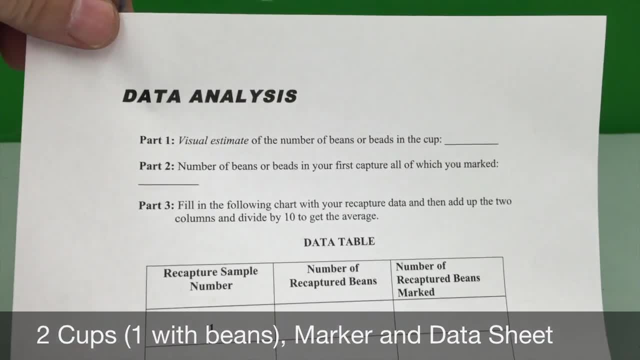 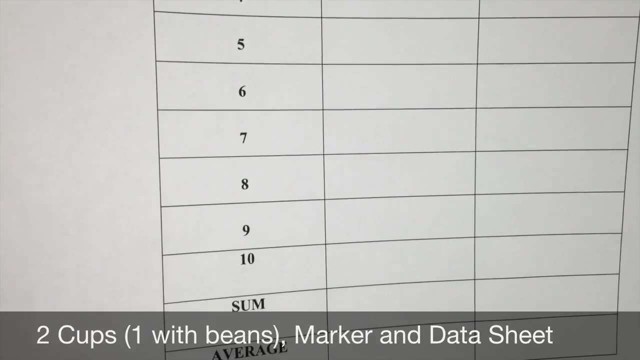 As far as the data sheet is concerned, it looks something like this: The data sheet that we have is in your packet and we're going to do 10 samples, so we're going to go out and collect 10 different collections on this particular lab, so make sure you assemble that before you start. 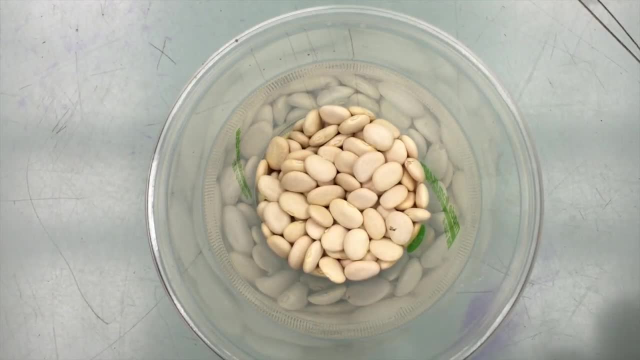 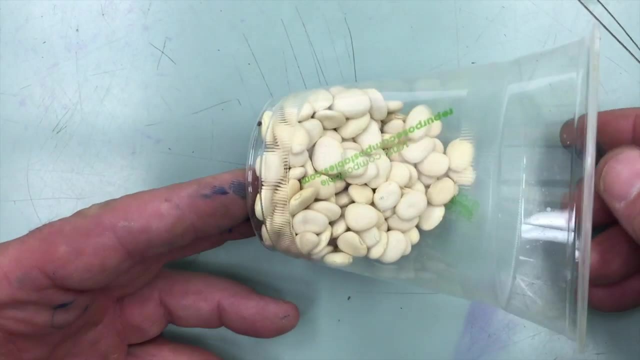 We're going to go ahead and go through the procedure so that you know what to do. Obviously, I would suggest you read the procedures first, as a group, so that you understand what's happening. So, anyway, if you take a look, our beans are filled up This one. 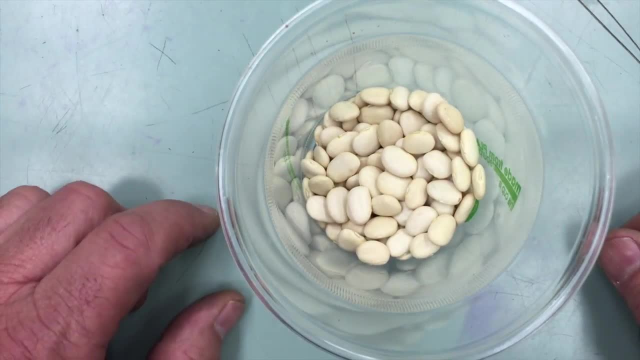 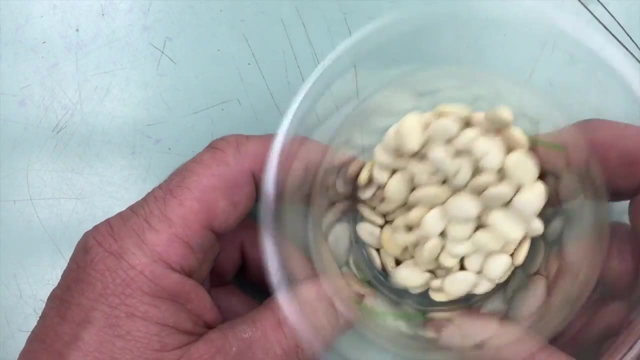 is about a quarter of the way full. I would recommend about half. One of the first things you do is you need to take a really close look at the beans and give a visual estimate for the count. You need to write that down. so I'm going to bring in our sheet. 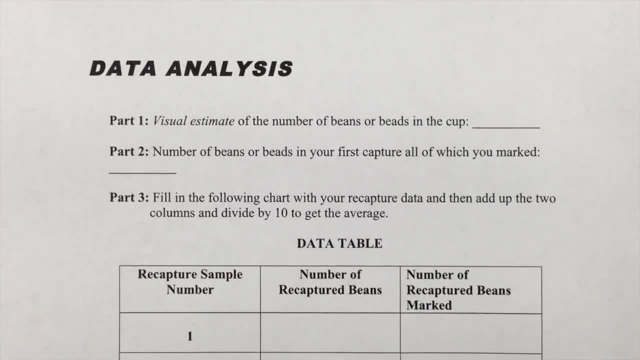 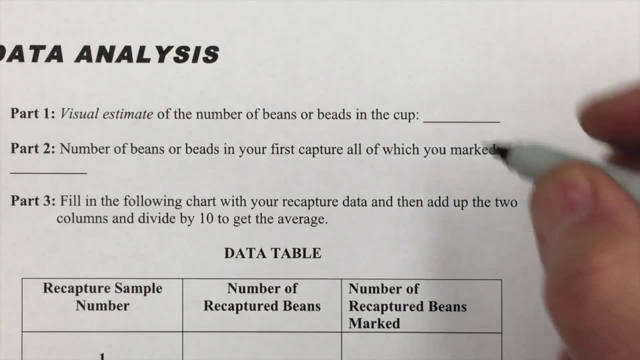 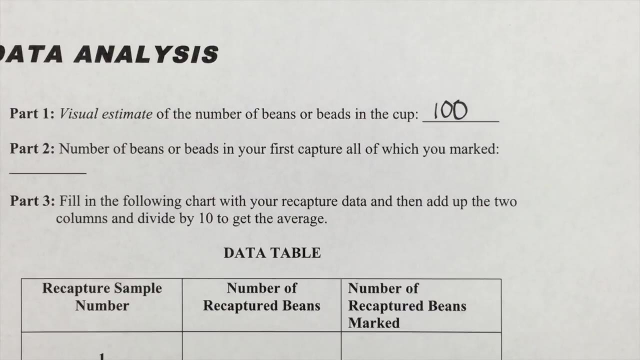 right here. and then it says on part one. it says: go ahead and do a visual estimate of the count of beans- and I'm just going to say a hundred, That's going to be my guess- and the number of beans or beads in the first capture in which you mark. 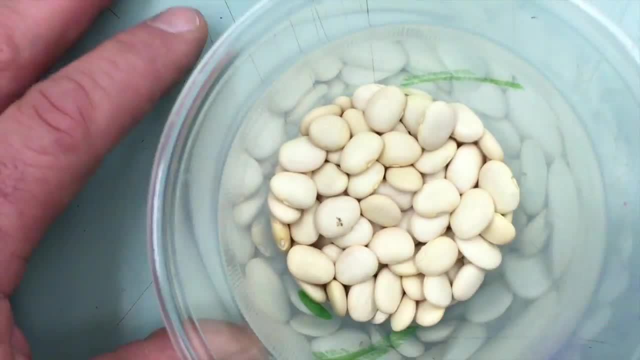 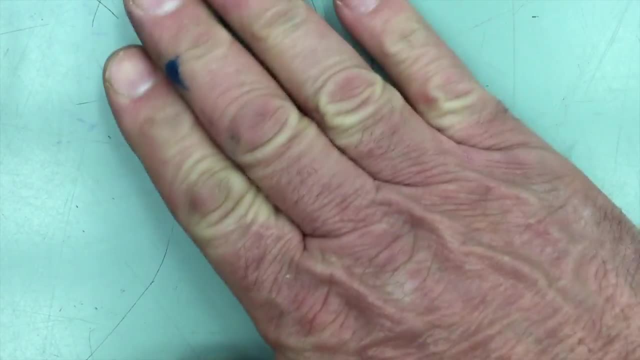 So let's go ahead and do that next. So to do that, what you'll need to do is you're going to kind of put your hand in the cup, dig out a few and then put it on the table. You don't have to get a whole big handful. 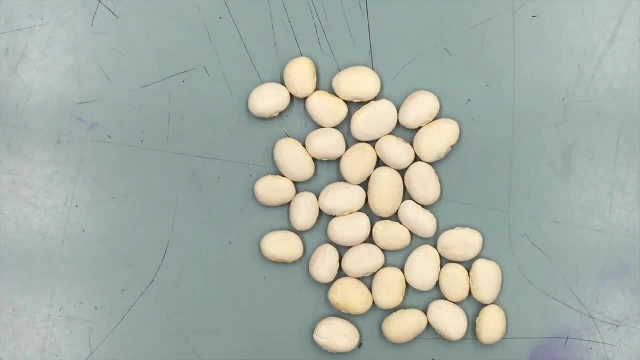 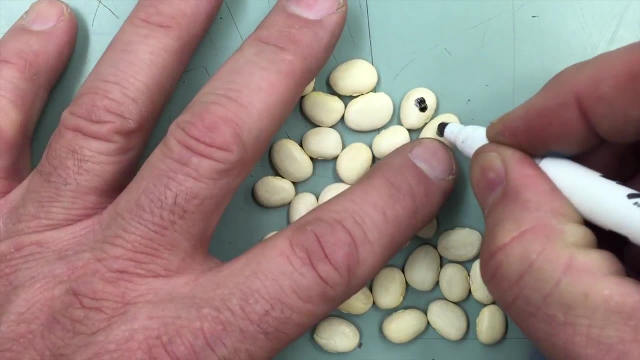 You just need to go ahead and do it. These are the ones we're going to mark, and we're going to go ahead and mark those, and you're going to mark them all by putting a big dot on it, just like that. 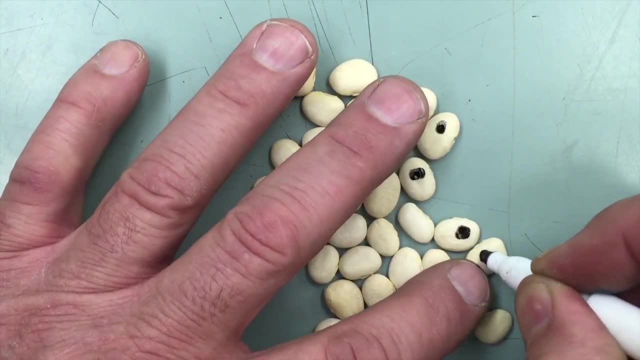 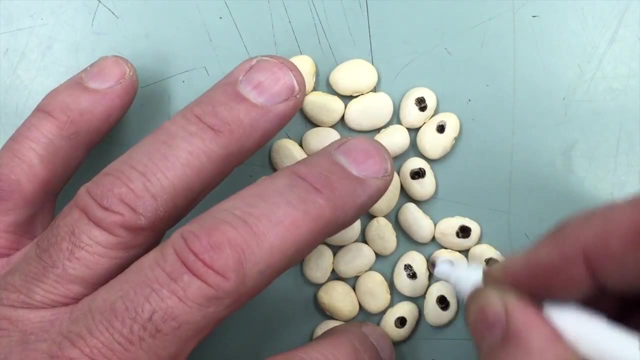 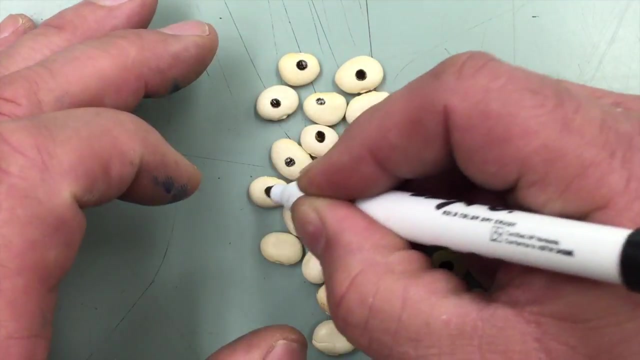 Now you can put them on both sides. As a matter of fact, the instructions recommend you do that. That way you can see it much easier. So I'm marking all of these just like that, And as we do that, it's kind of like ear tagging them. I'm giving them a thin tag or something like that. 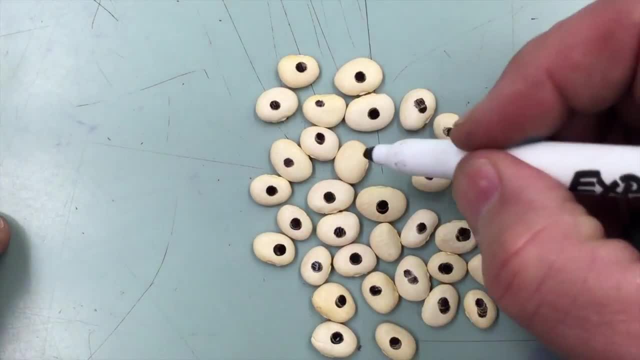 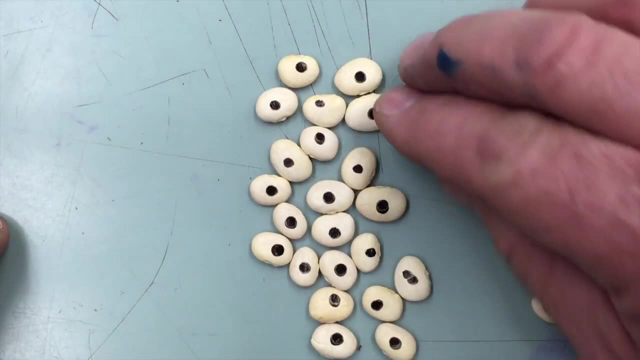 Now what we're going to do is count them really quickly. I forgot one right there, See two. two of them right, One there, one there, And we're going to go 2, 4,, 6,, 8,. 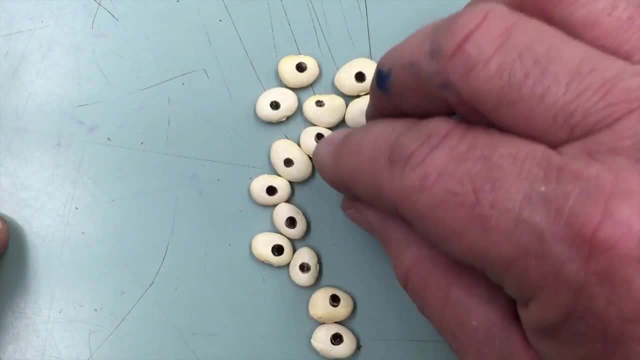 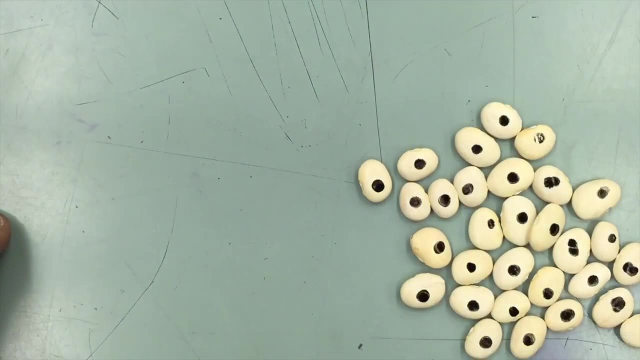 10,, 12,, 14,, 16,, 18,, 20,, 22,, 24,, 26,, 28,, 30,, 32.. So we have 32 of the ones that are marked. Some of those you saw there were unmarked. 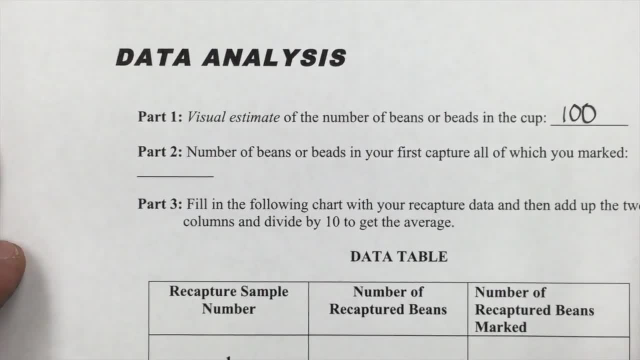 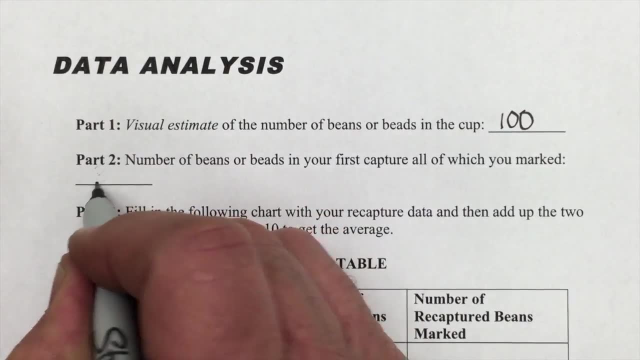 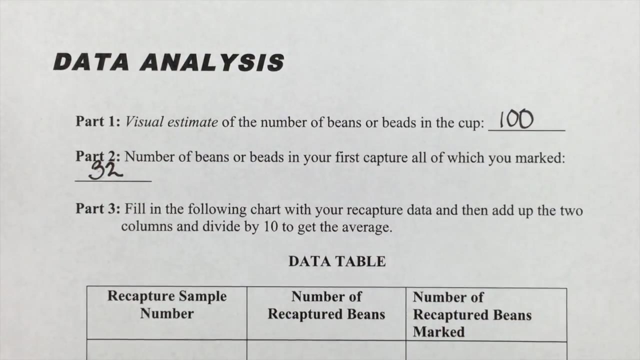 That was because they flipped upside down. So we're going to look at this. I'm going to put number of beans and you first capture all of what you marked. We're going to put 32.. And again, I'm working with about half the amount that you should, so I'm going to keep that in mind. 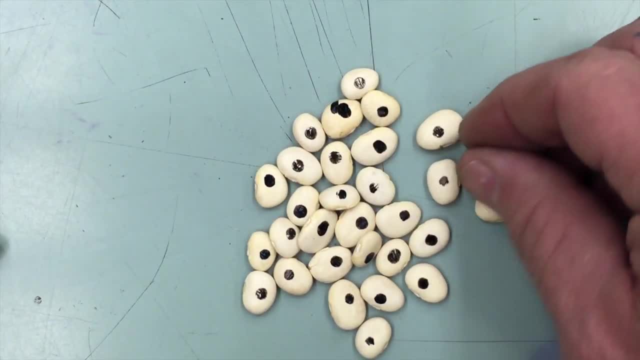 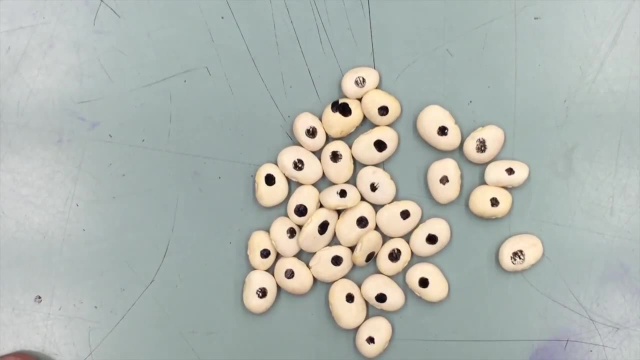 What I've done is I've checked to make sure we have marked them on both sides so that every one of these beans which represents a small animal we have marked so that we can find them again. So at this particular point in time, we're going to take all of these beans off. 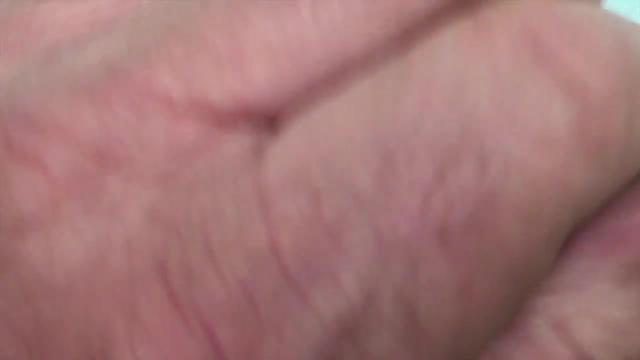 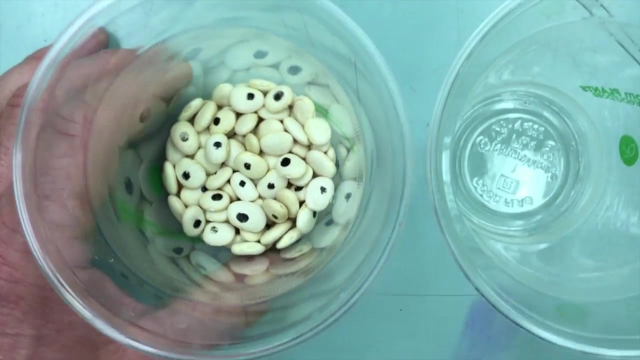 And we're going to pour them back into the population. And when you do that, that's where the other cup kind of comes in handy. What you're going to do now is you're going to go ahead and mix them together, Give it an ample opportunity to mix in the population. 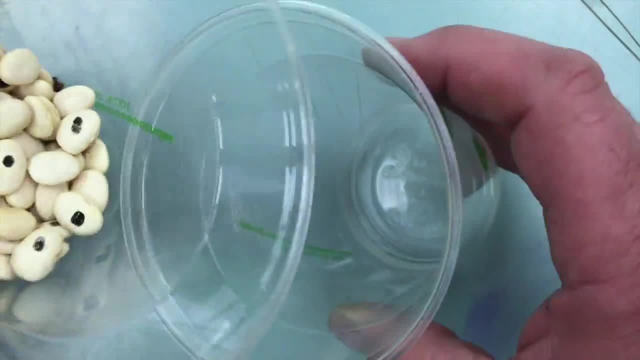 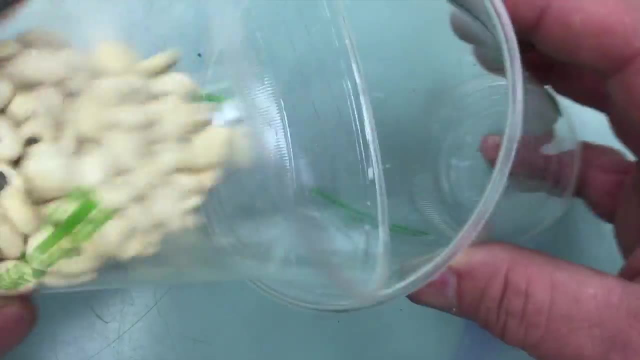 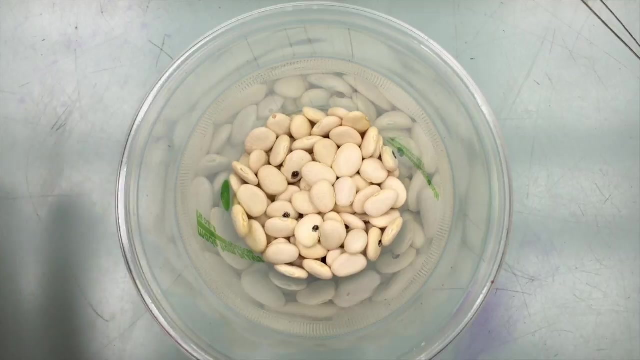 Remember. part of the premise here is that when these particular animals give enough time, they then slowly redistribute themselves evenly throughout the population. That's what this represents, Now that you've mixed up the beans enough so that it represents all of these particular animals redistribute themselves in their environment. 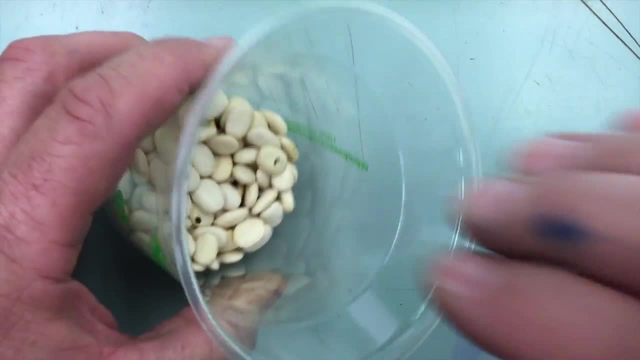 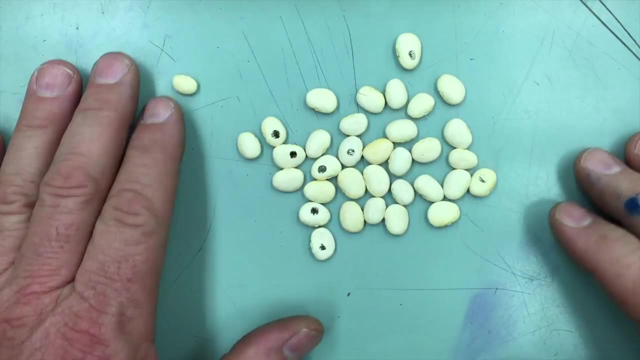 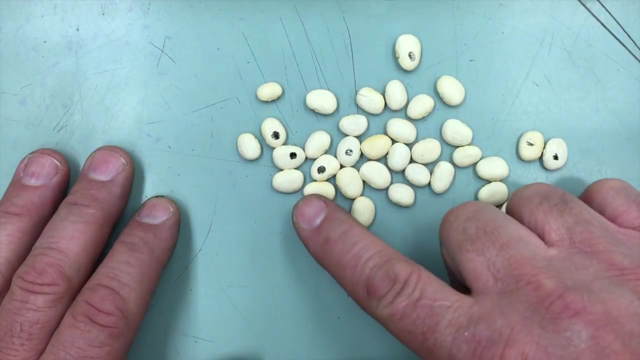 we're doing a series of recaptures. How you do that is just take a handful of beans, drop it down, and then what you want to do is you want to count all the marked beans, like in this case: there's one, two, three. 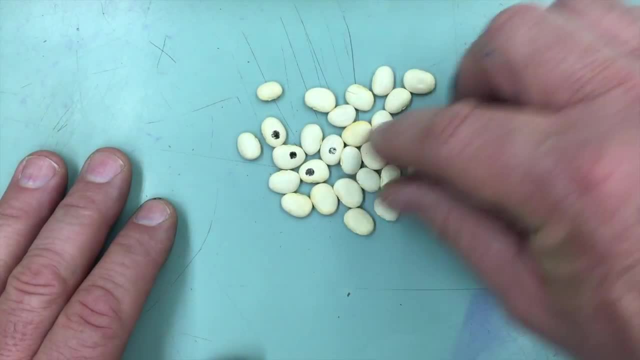 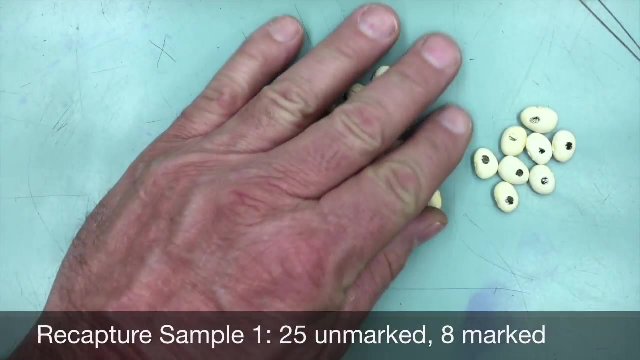 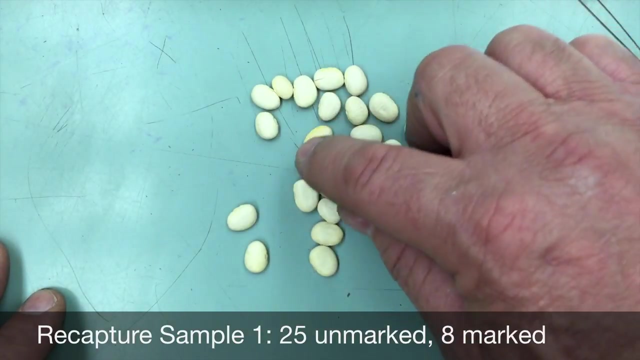 four. let's put these back over here. there's four of them, five, six, seven, eight. So there's eight recaptured beans, And then you have one, two, three, four, five, six, seven, eight, nine, ten, eleven, twelve, thirteen, fourteen, fifteen, sixteen, seventeen, eighteen, nineteen, twenty, twenty-one, twenty-two, twenty-three, twenty-four. 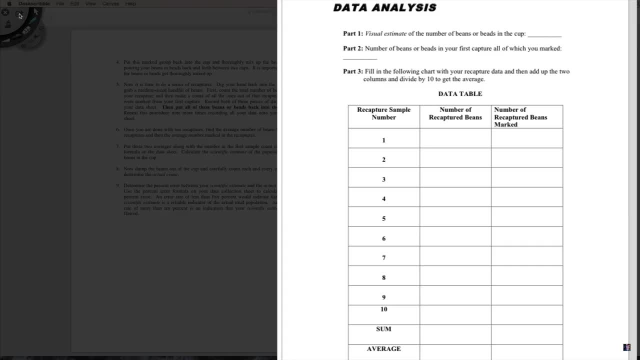 As you're pulling beans out for each of the recaptures, you're putting them on this data sheet And before you actually do the first one, what you really want to do is you want to estimate just by visually looking at the cup. 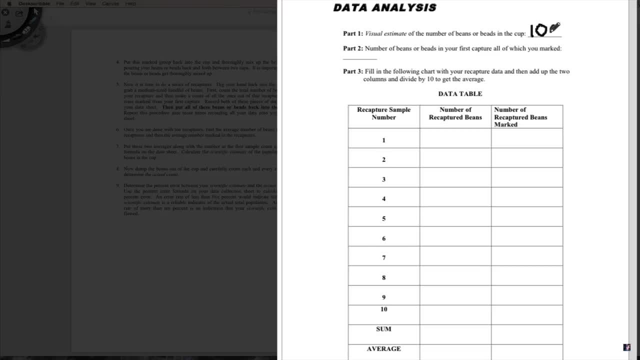 And for the cup that I had, I'm going to say it looks like about 100 in there. That way we can compare what our visual sense to say versus what the actual count says. And also on the first capture we actually marked 32.. 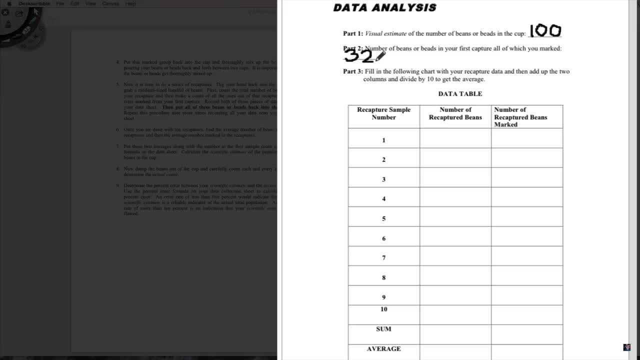 And in the second run we really captured 20 beans. So we're pretending they could be fish, they could be birds, whatever they might be, but they're animals, But the beans just kind of represent that animal population. So when we take a look at our first recapture, we had 33 total beans that we collected. 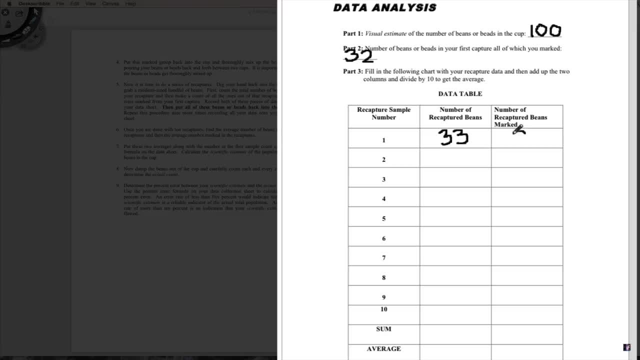 And of those 33 of them, eight of them were marked. In the second run we recaptured 20 beans, Or birds, or fish or amphibians- whatever you're trying to capture- with three that were marked or tagged. And then we went to our third one, which was 30.. 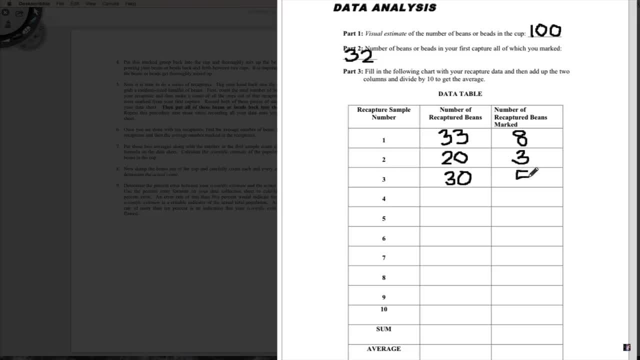 And we caught five, or actually we had five that were marked. So that's what those data looks like. So we continued out until we went all the way to the last one And in the last recapture we had 43 total beans or animals recaptured. 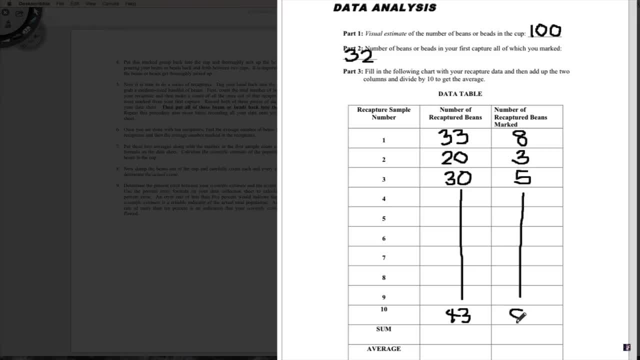 And of those 43,, eight of them, eight of them were marked And if we were to summarize, or if we were to add up all of the 10 runs, we'd have 362 total beans or animals caught. And to get the average we're going to divide that by 10, because there's 10 runs. 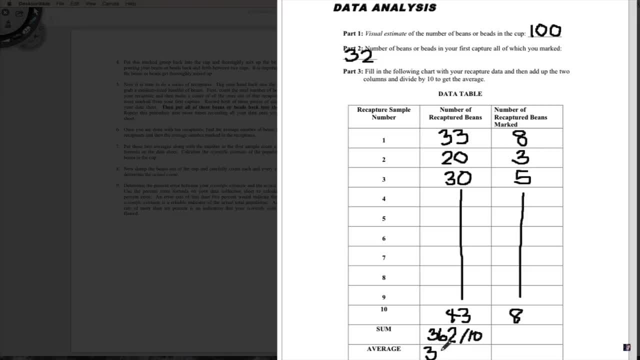 So we got an average recapture rate of 36 beans, 36.2 to be exact, On the actually marked recapture side. when I added them all up, I got 71. And then, of course, we divide that by 10.. 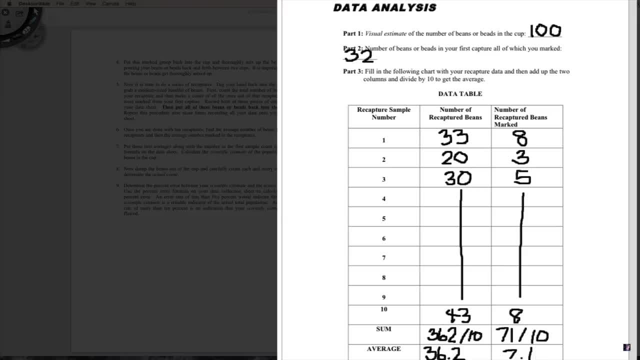 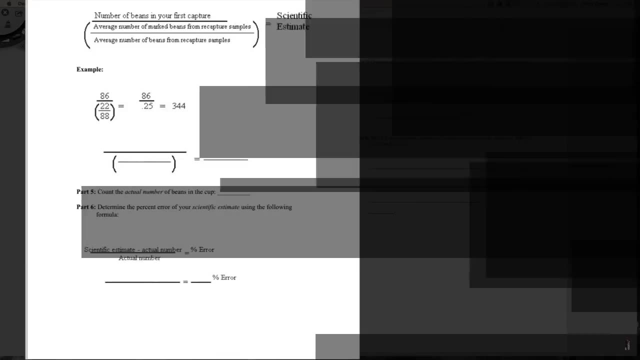 And that would get an average marked capture of 7.1.. Or essentially seven beans that were marked when we collected them. Now we're going to take these numbers next. And now we're going to The analytical part of Once you have all your data recorded in your data table. 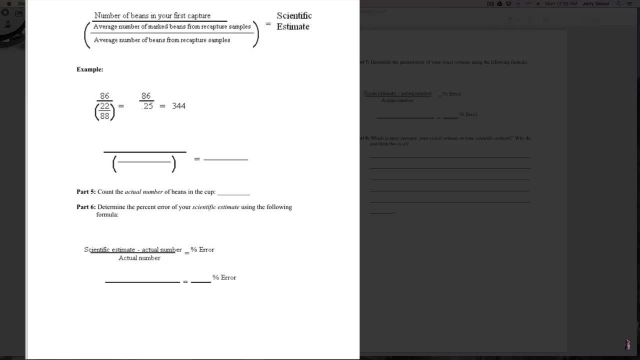 now it's time to figure out how many individuals do we have in this population. That's what all of this data collection was really about, is how many animals are in the population without having to count each and every one of them. So one of the first things we did is we looked at how many beans we made in our first capture. 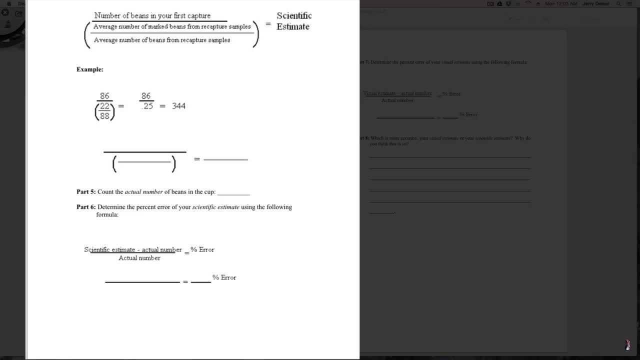 In other words, we captured 32 beans. if you remember correctly And you watched the video, Then what we did is we marked each one of those beans, So we have 32.. So our first sample was 32.. And we marked all of those 32.. 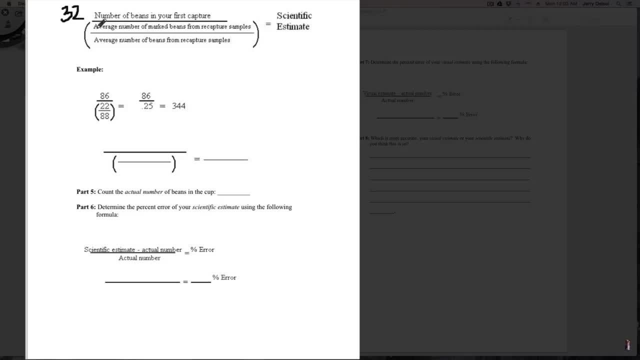 And then we turned them back in with the rest of the population. The average number of beans, if you remember right, it was 7.1.. We had a total of 71 marked beans. We added them all up after 10.. 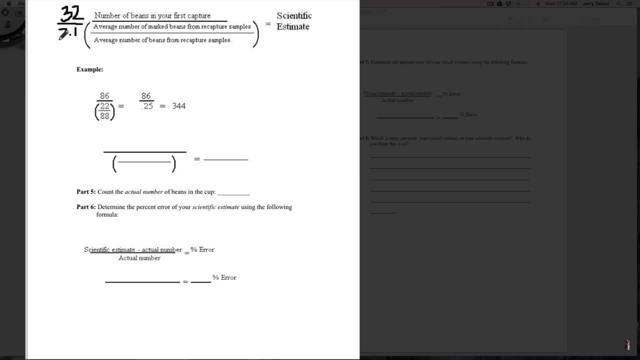 That was 71. So the average is given an average of 7.1.. And we did the same thing for just the number of beans that we recaptured. There was 362.. We divided that by 10. And we got 36.2 beans. 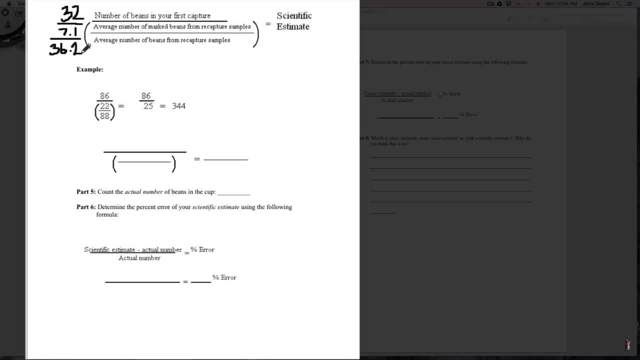 Now, remember, the beans are analogous to animals, things like birds and fish and that sort of thing. Once we get all of this mess now, we're going to turn it into something that we can kind of understand. So we're taking the 32,. 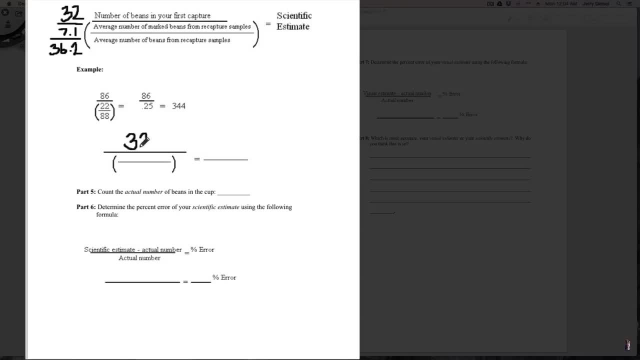 total number of beans that we marked, And that's 32 right there. Average number that we recaptured that were marked was 7.1. And then the average number of marked and unmarked beans that we have per recapture was 36.2.. 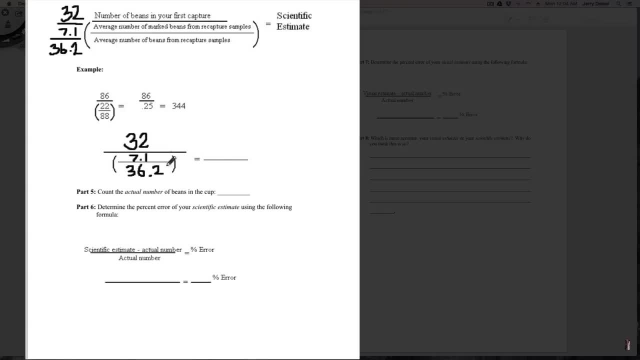 And when we did all of the math there we had, when we divided this, we got .196.. .196. And we divided that into 32. And according to the scientific estimate that we have, that came out to 163.2 individuals. 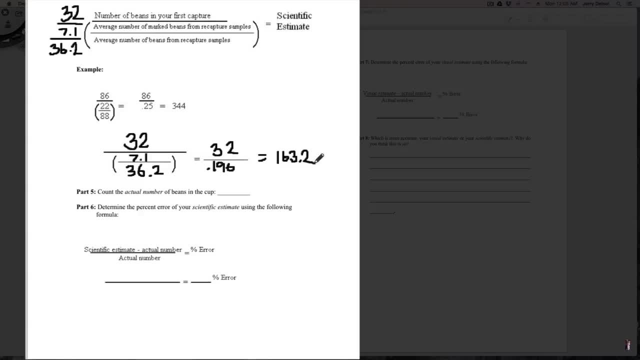 So we can just call that 163. But if you want to keep it clean, that would be it. And then 179 is what we got when I actually counted. We have the actual number. I'm going to count beans Now in the real, when we're out in the real world. 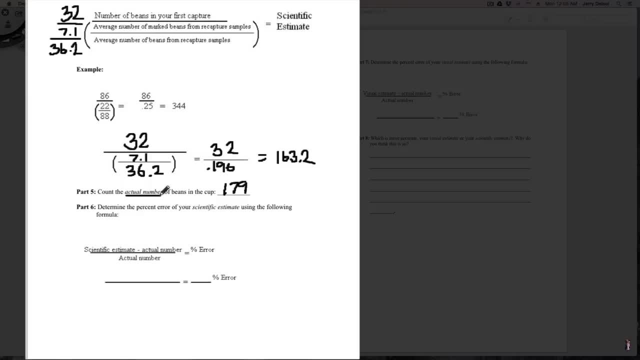 we probably can't count them all, So we have to kind of rely on a method. And if this is the method, it looks like it's pretty close. But let's run a percent error test on it to see if indeed mathematically it's close. 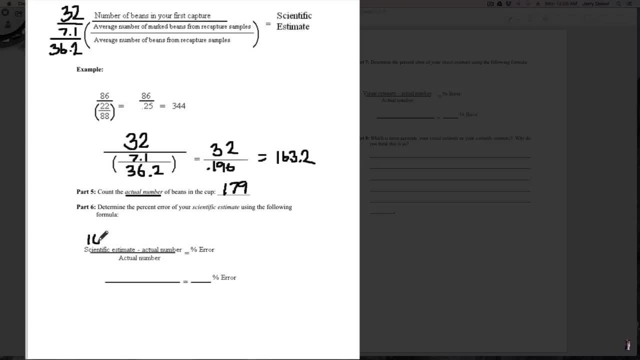 Scientific number is 163.2.. And we subtract that by their actuals 179.. That comes out to 15.8.. And then we divide all of that by 179. And then we'll get a percent error. Well, actually it's like a relative error.